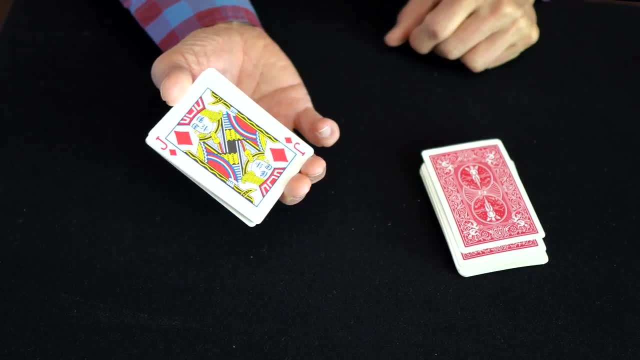 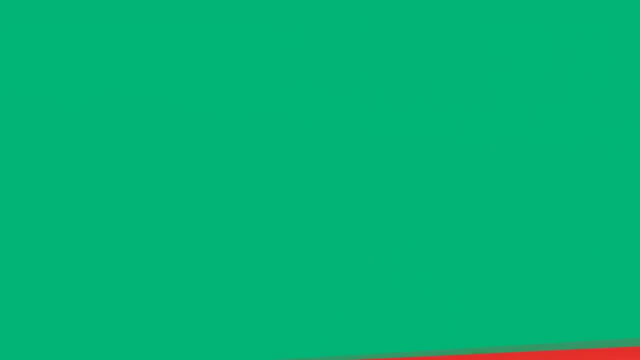 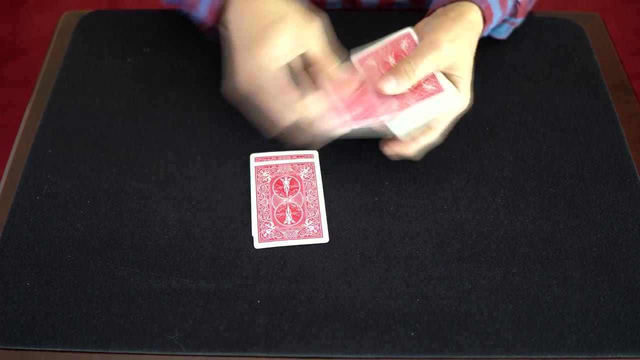 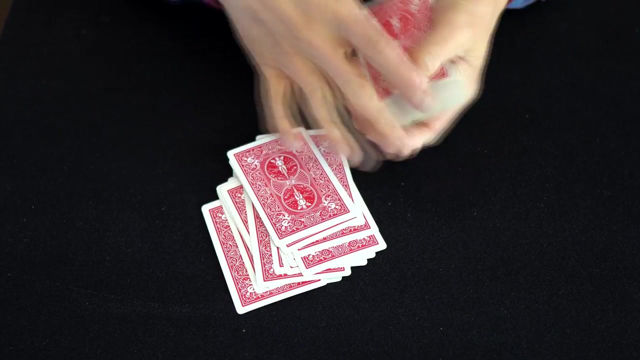 that you stopped on the Jack of Diamonds, and that would be correct. What I'd like you to do, please, is just say: stop, as I deal the cards onto the table Anytime you like. take your time Some time today. 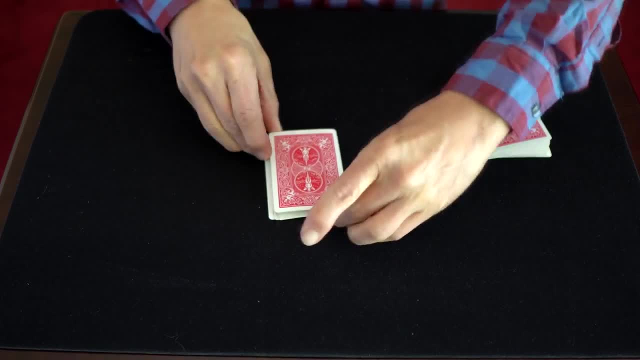 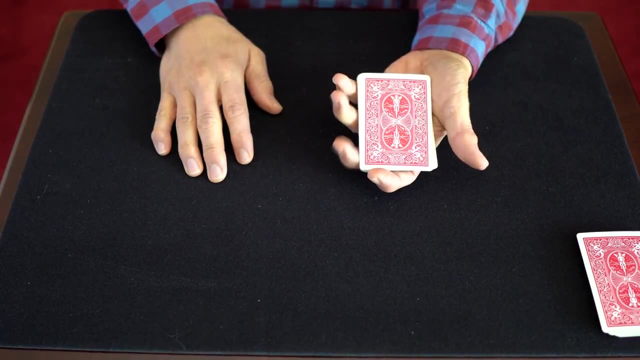 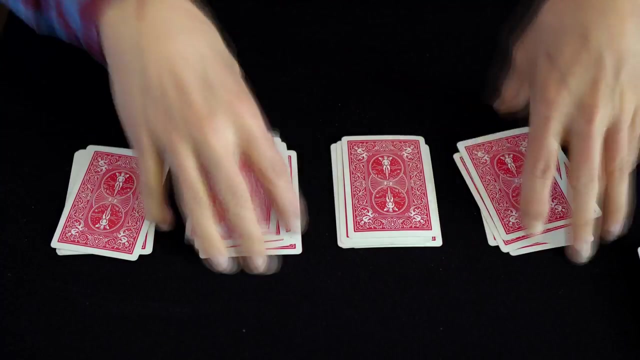 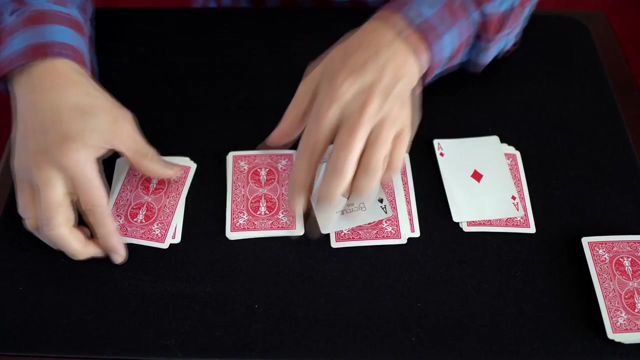 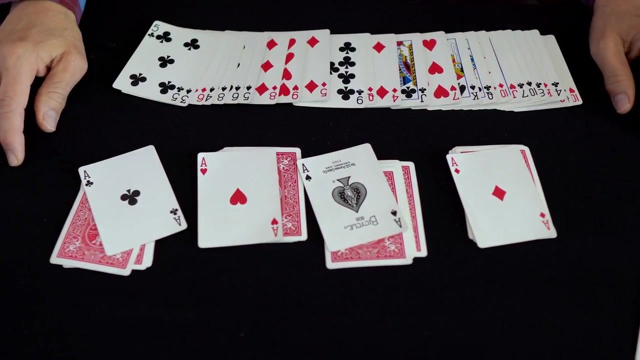 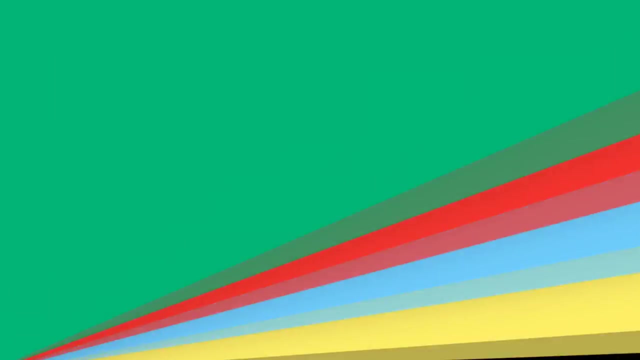 Was that a fair choice? Excellent, I'm going to deal this into four piles. Now, you had a free choice, right. Let's see how you did. Four Aces, Nicely done. I want to tell you a story about my favorite cards, the Jacks. 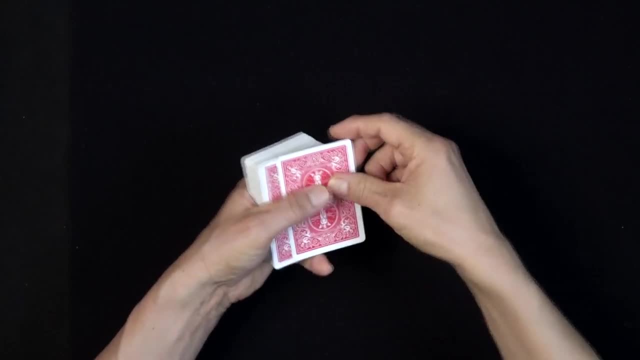 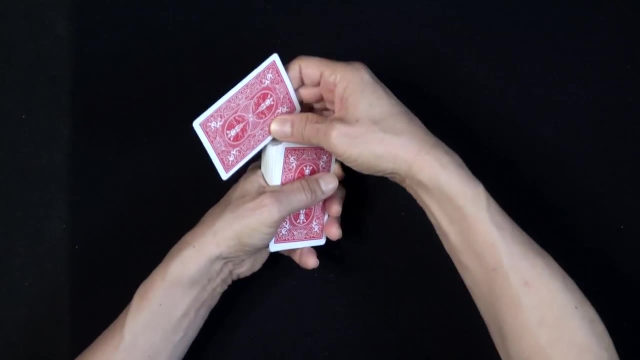 You see, they went on a hike one day and unfortunately they got lost. One Jack got lost in the bottom third of the deck. Second Jack got lost in the middle, And the last Jack got lost in the middle And the last Jack got caught somewhere near the top. 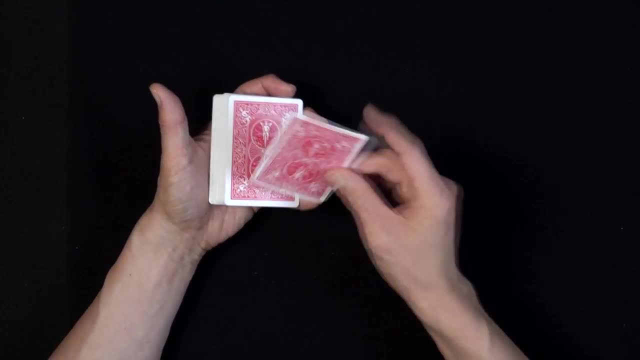 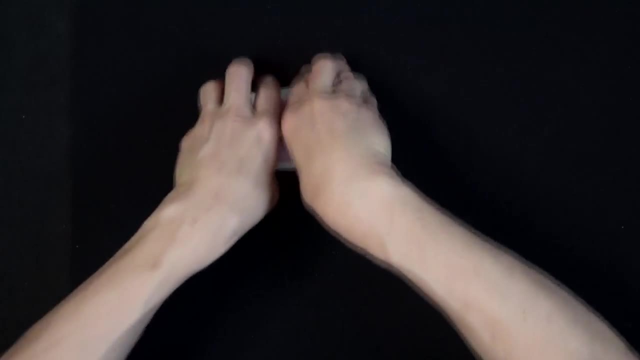 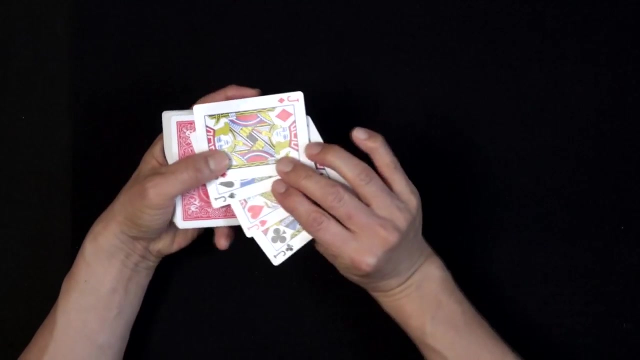 They were separated. The last Jack stayed back at home base. But this is a magic trick, Because all you have to do is give a little cut here, a little mix, and magically a snap of the finger will bring back the four Jacks right there. 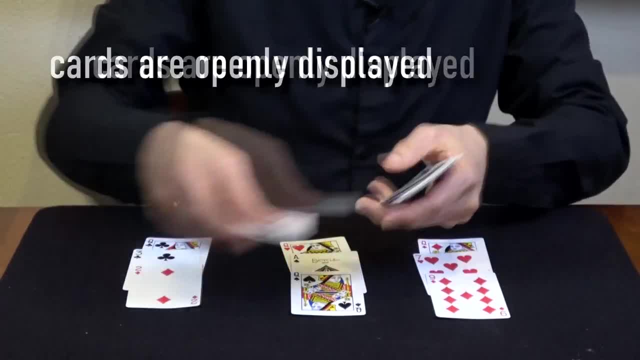 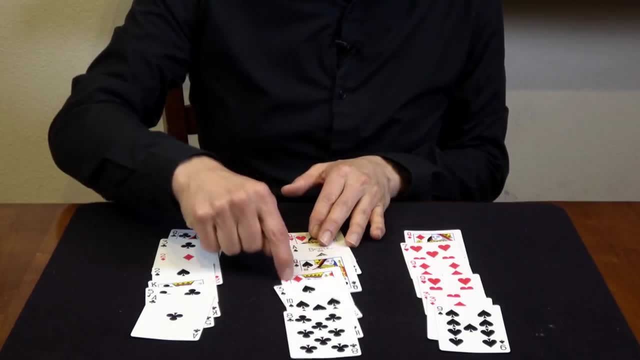 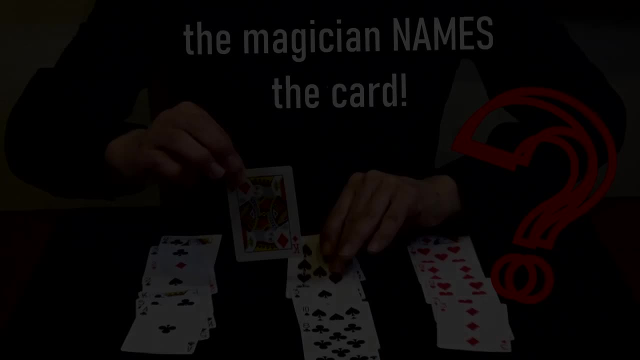 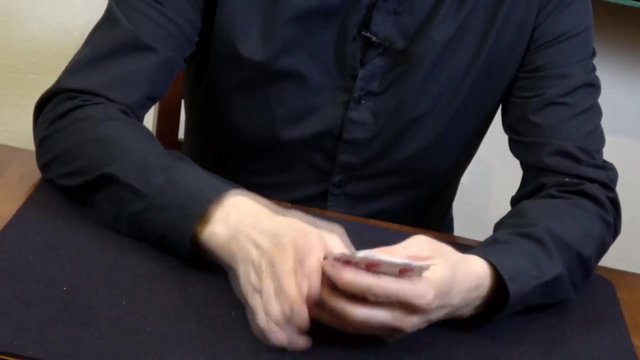 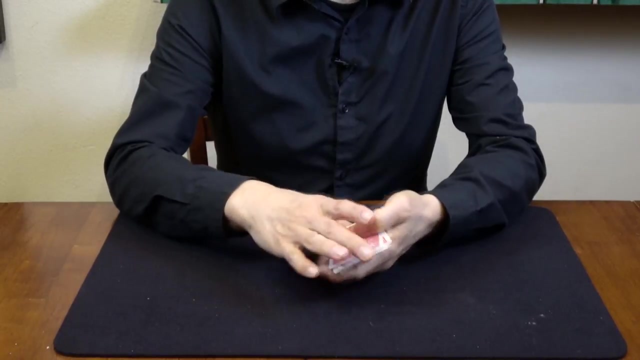 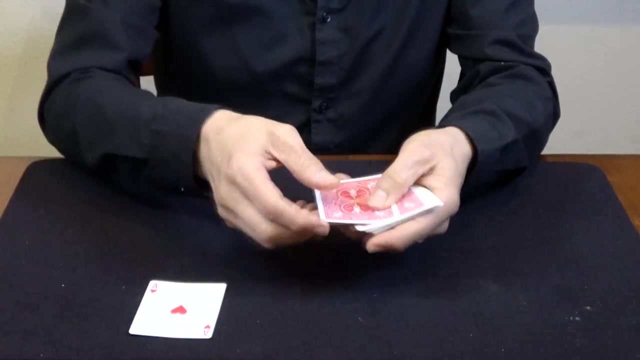 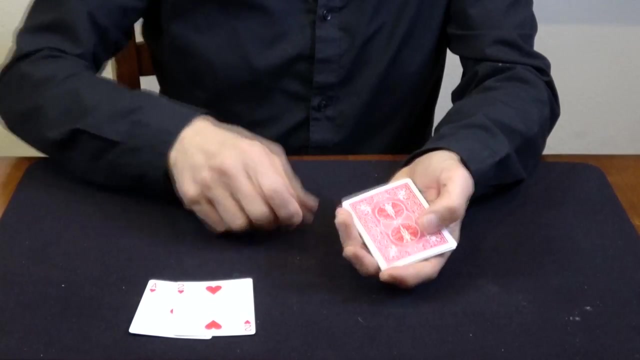 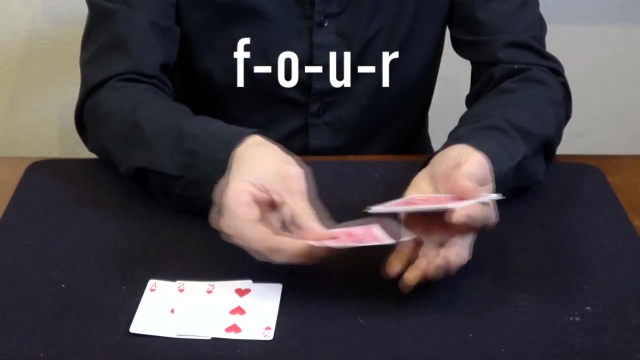 I have here some cards And we're just going to spell and see if we can go to every card. So we're going to start at the bottom with an ace. so let's spell ace A-C-E and that should bring up an ace: 2-T-W-O, 2, 3, T-H-R-E-E, 3,, 4, F-O-U, 4,, 5,, F-I-V-E. 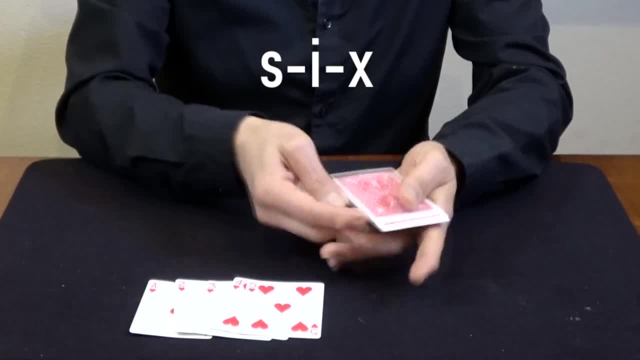 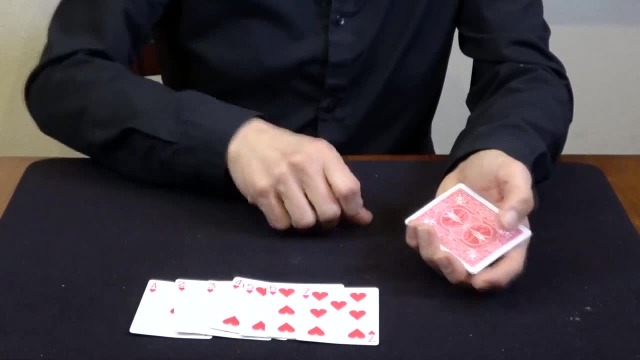 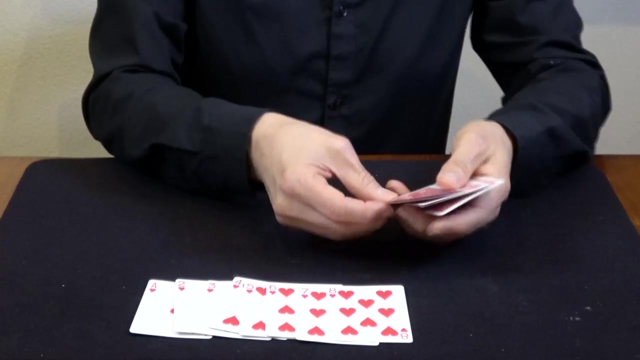 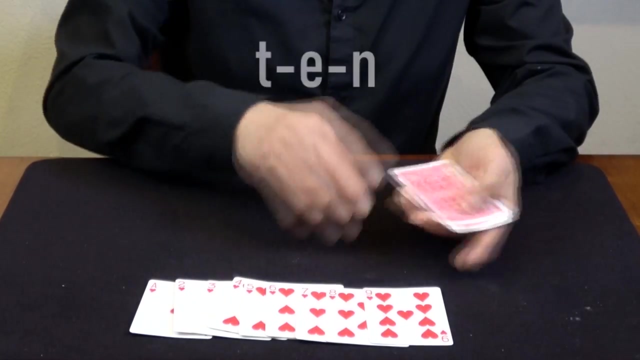 5,, 6, S-I-X, 6,, 7, S-E-V-E-N, 7,, 8, E-I-G-H-T, 8,, 9, N-I-N-E, 9, T-E-N-10,, Jack J-A-C-K. 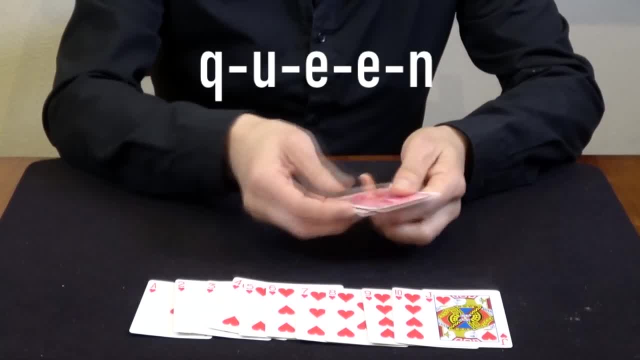 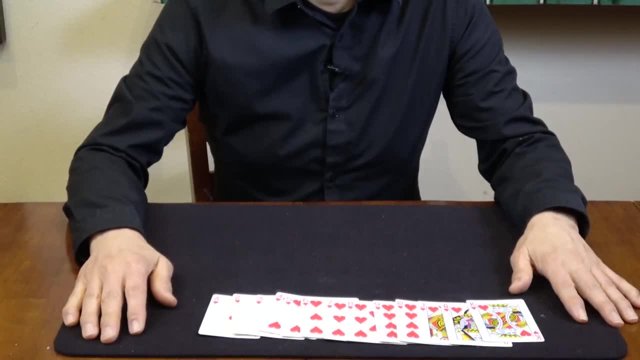 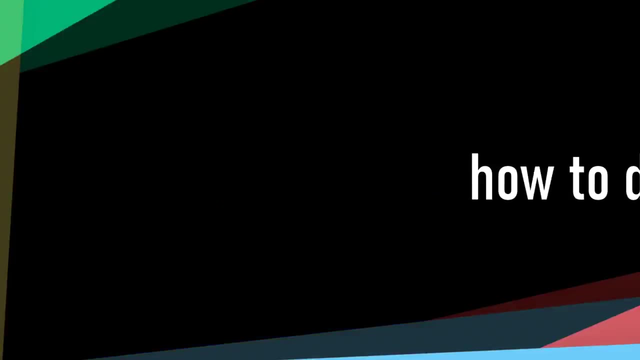 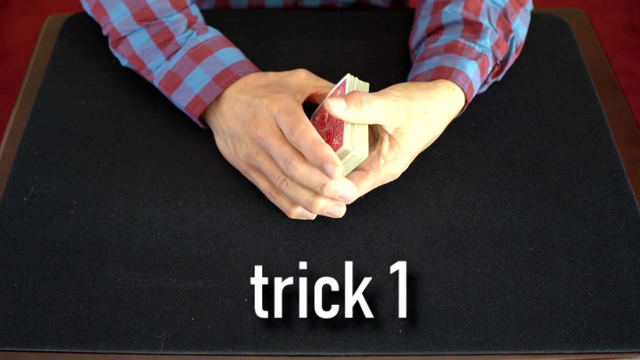 J-A-C-K. Queen, Q-U-E-E-N. Queen and the King. and there we've done it. we've spelled to every card, one by one. Here's how to do the trick, a classic that I think every kid learns. 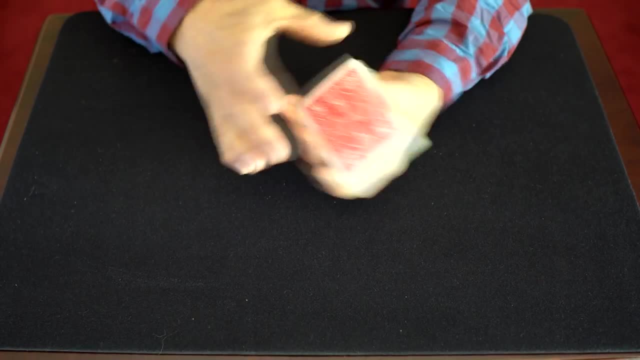 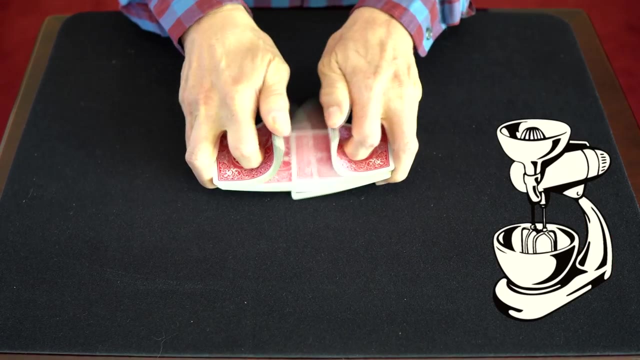 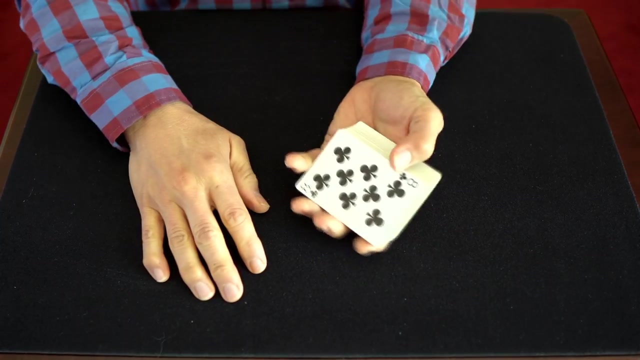 Along the line and it's a fast, easy trick. All you need is an ordinary deck of cards. hand the deck to the spectator. they get to mix. Now, when the kids get the deck back, tell the spectator you're memorizing the deck. 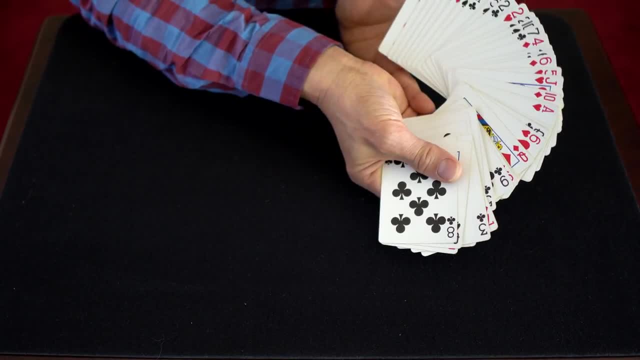 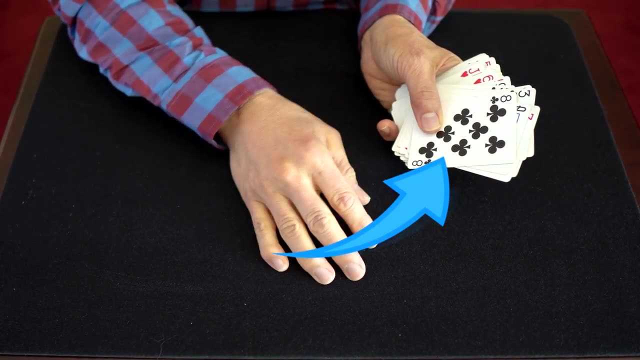 The deck is actually mixed, and so you look like you're memorizing the deck. however, all you're doing is looking at this bottom card. Whatever ends up at the bottom, That's your card that you remember, and in this case, it's the Eight of Clubs. 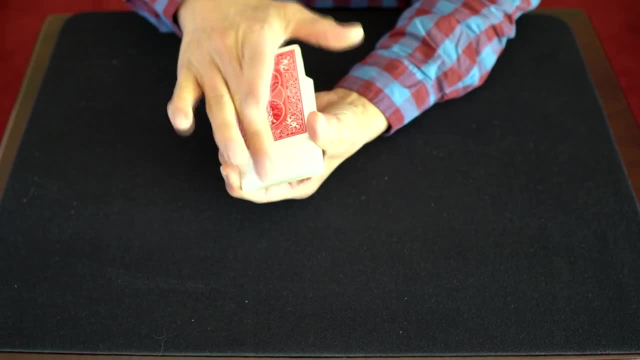 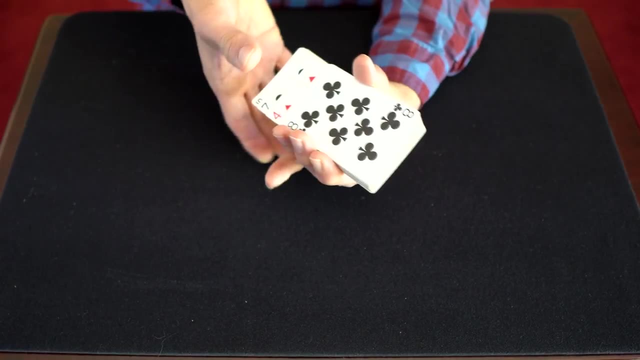 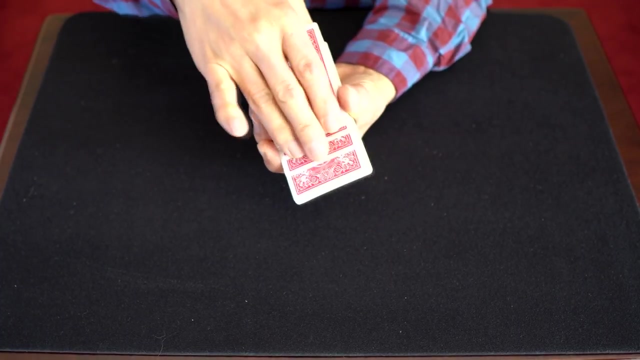 So here's how it works: As you move the cards down- and it is a free choice to say stop. what happens underneath is what happens is your thumb pulls back the bottom card. So underneath all this, here, while this is going on, I actually have this bottom card. 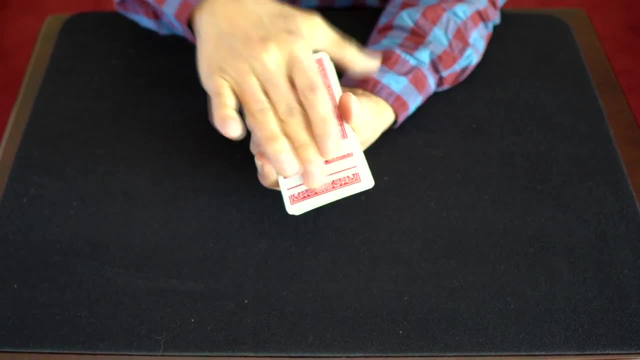 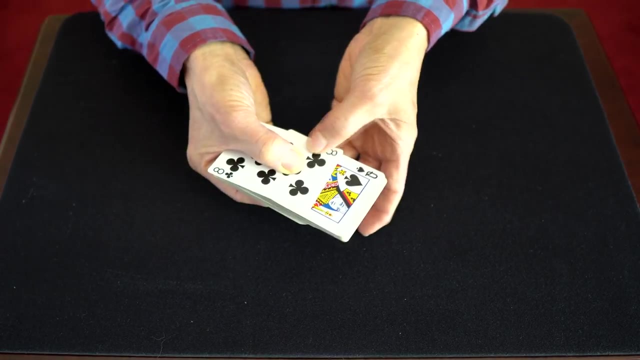 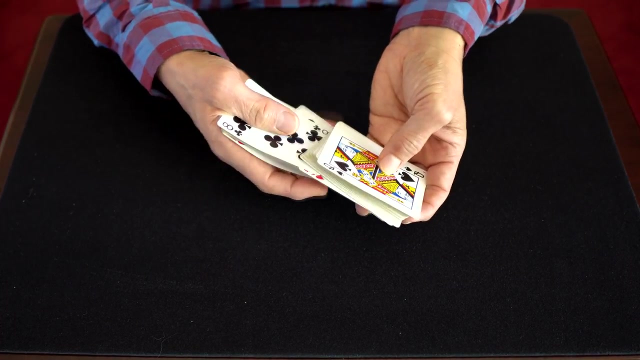 pulled out. Now the spectator says: stop wherever they want. And what happens here is on the bottom. my thumb is going to remove this bottom card, the Eight of Clubs, with the rest of the pack wherever they say stop. Just like that. that's what happens underneath the action and then when you pull it out, 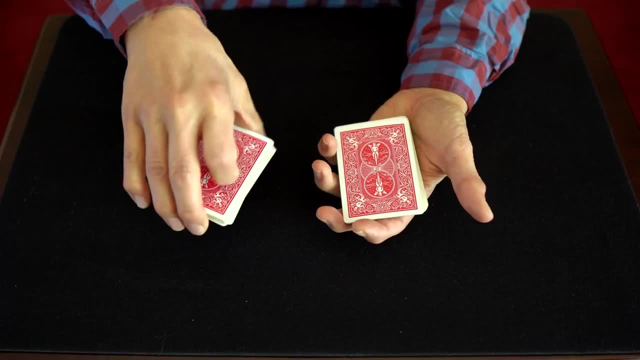 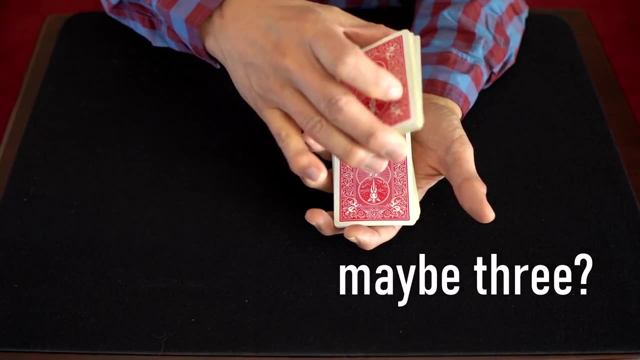 you say: let's see, I remembered the deck and you stopped on the Eight of Clubs and you can show it and you can repeat this. I wouldn't do this more than two times, maybe three, because spectators will be really watching. 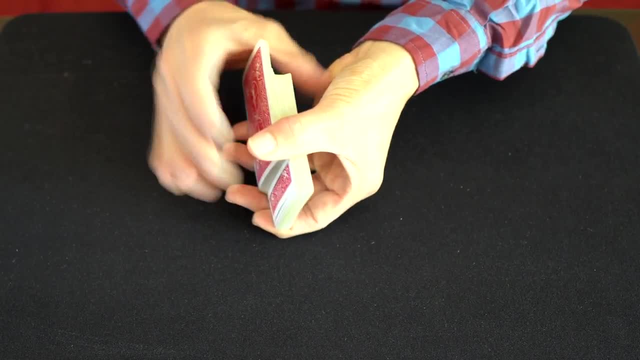 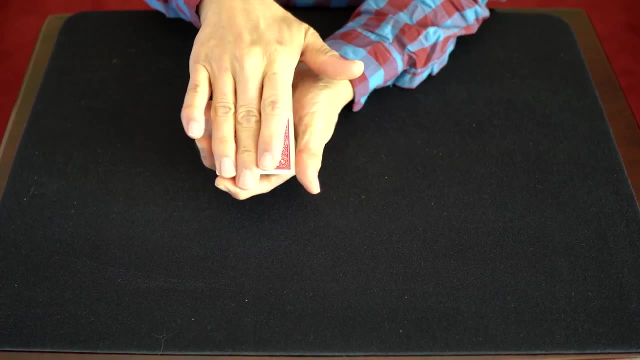 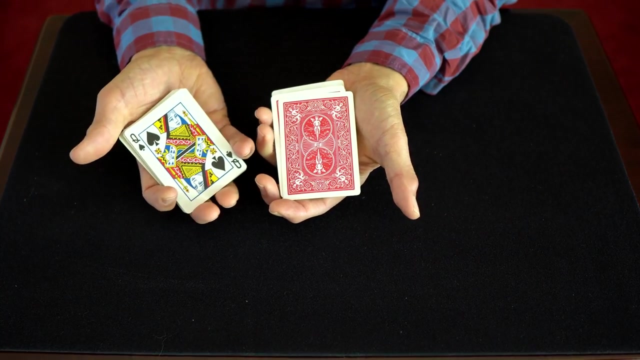 And just watch that angle. you don't want to be doing it like this and then having spectator C pull the card out. with the rest, you want to keep the deck towards the spectator like this and the thumb underneath, and you can always pull out that bottom card as if. 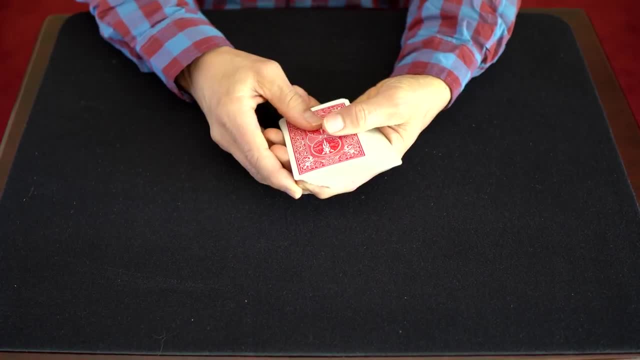 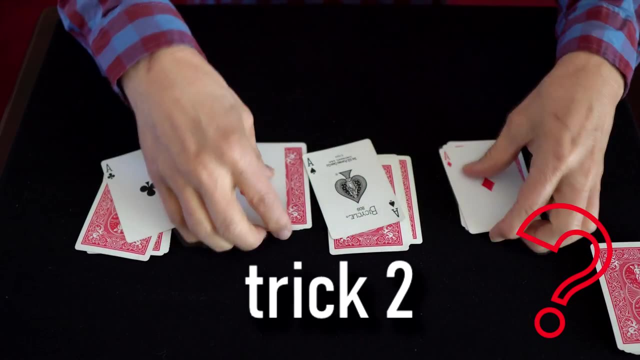 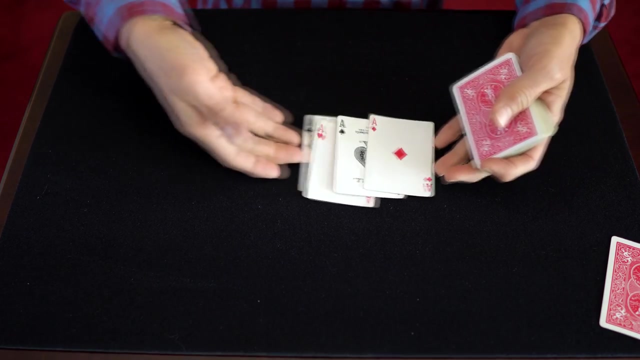 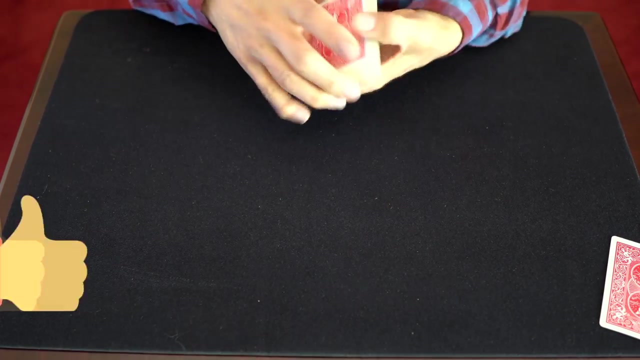 you had memorized the entire deck. What you'll need for this trick is an ordinary deck of cards and the Four Aces. Just remove the Four Aces ahead of time. place them on top of the deck. You're ready to go. 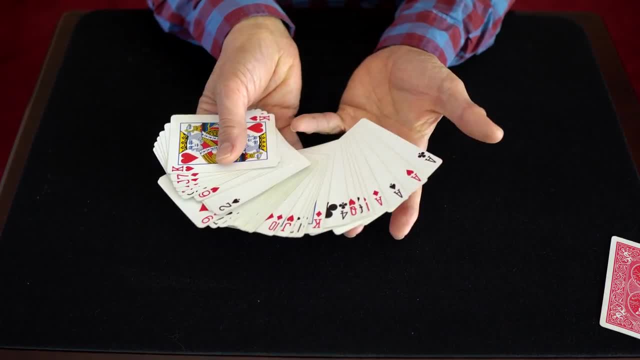 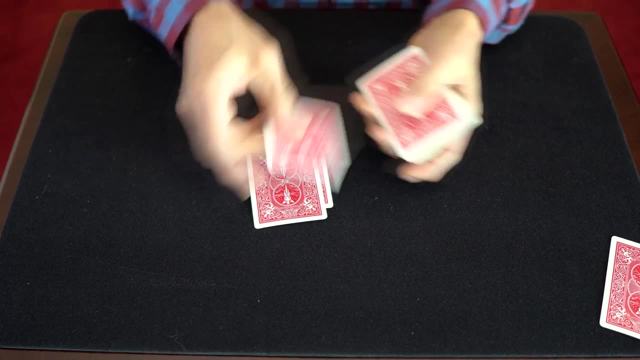 Bring the cards out. you just show that they're all different, Don't show the back four- over here, Spectator doesn't know about the Four Aces- and deal onto the table. Now what happens is the Four Aces end up at the bottom of this pile. 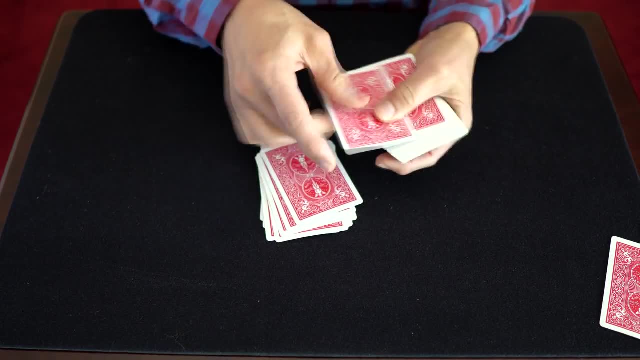 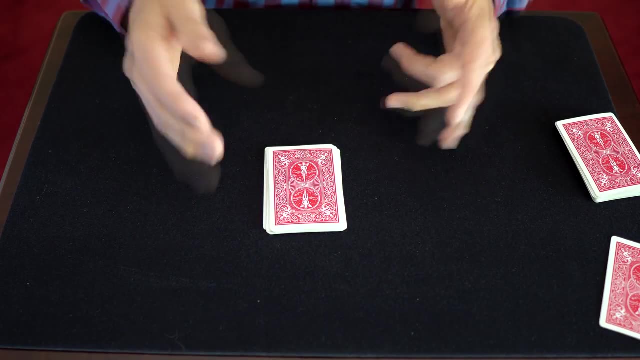 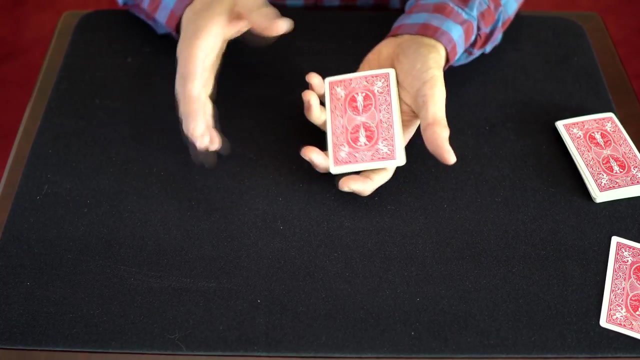 Spectator doesn't know that. Spectator just says: stop at any time, Move the rest of the cards. Notice that I asked a question here because that gives us a little space, because the spectators don't know about this, but it gives a little misdirection when you ask: was it? 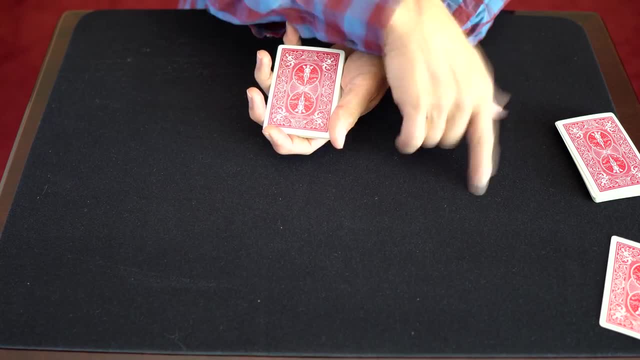 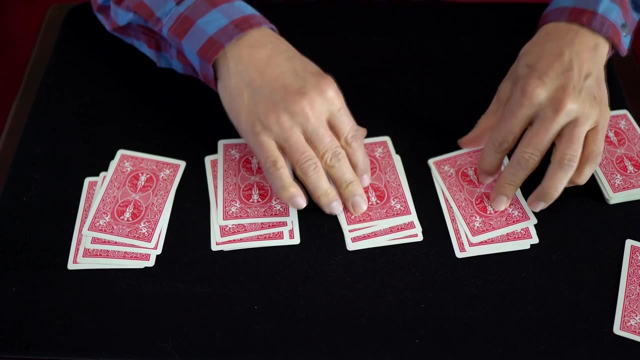 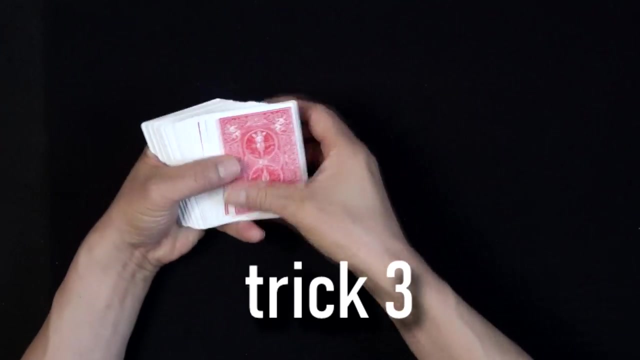 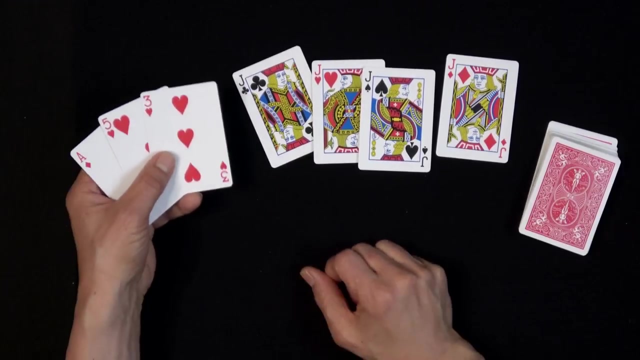 a free choice. Now, just deal into four piles And, because of the setup, The aces are now on top of each pile. Here's how you perform the trick: Ordinary deck- And you just need your four jacks, four queens, four kings, whatever. 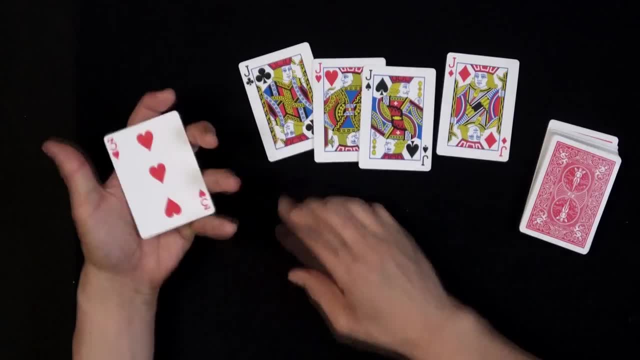 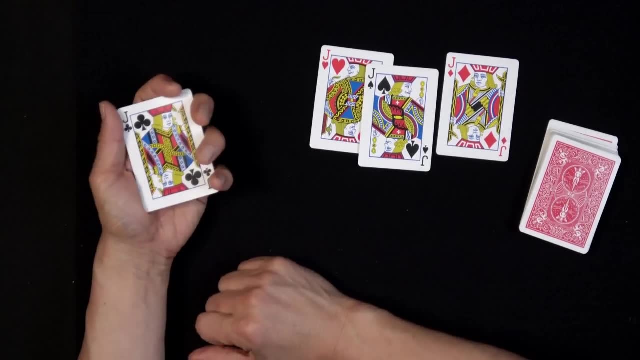 You want to use three and different cards here. You gather them up in your left hand And then you take one of the jacks, Place it on top, Line them up so it looks like a single card. Then you bring out these three and put them on top. 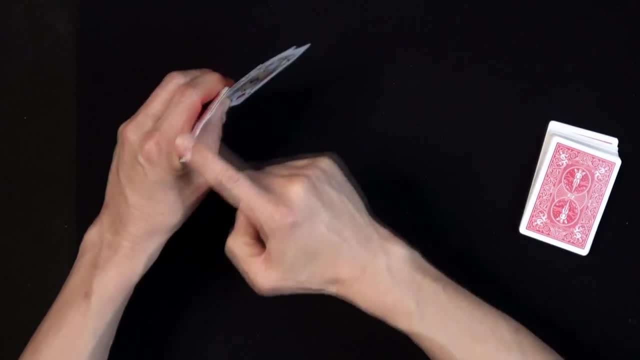 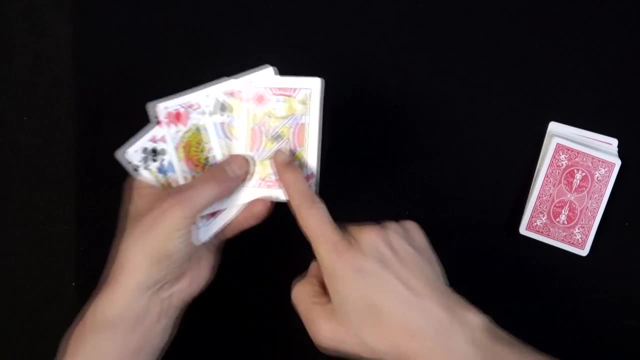 And you can just show these. As long as you don't turn it, they won't see the thickness. You don't want people to see this at an angle. You want them to see it directly looking on. So this looks like an ordinary card. 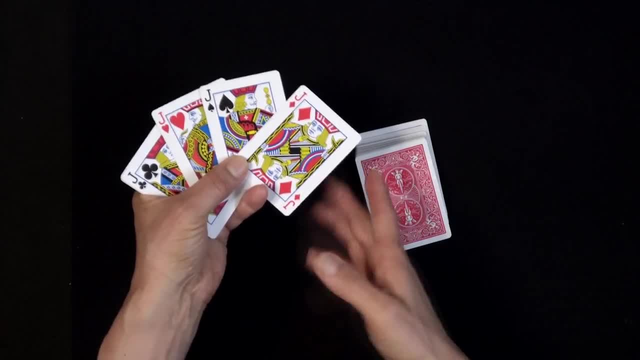 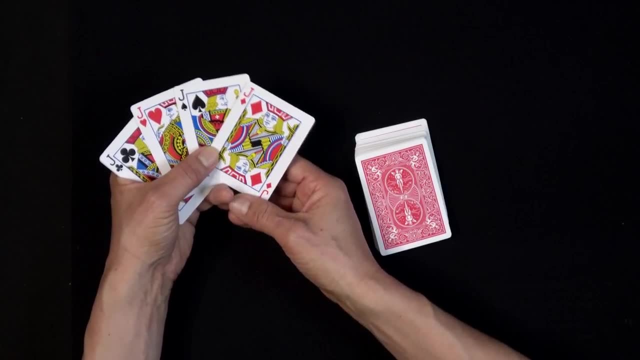 So you can show you have the four jacks And they go for a hike, They go for a walk. A lot of times in the beginning magic books, they call this four burglars. They get into a house or something or into a apartment building or commercial building. 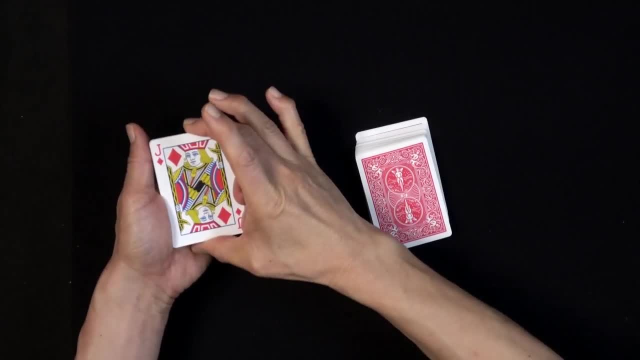 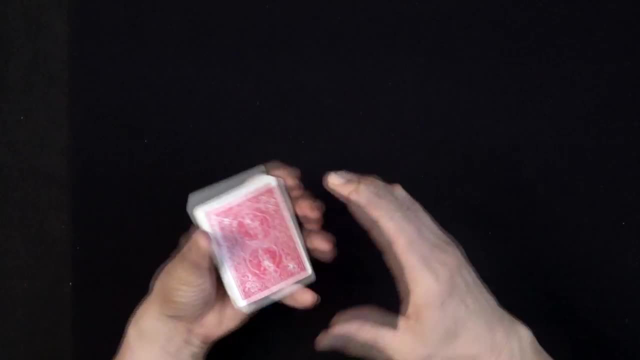 And they're on different floors of the building, But you just gather them up. People don't know about the three cards on the back. This goes on top of the deck And then you say they get lost. Whatever your story is, First one goes near the middle. 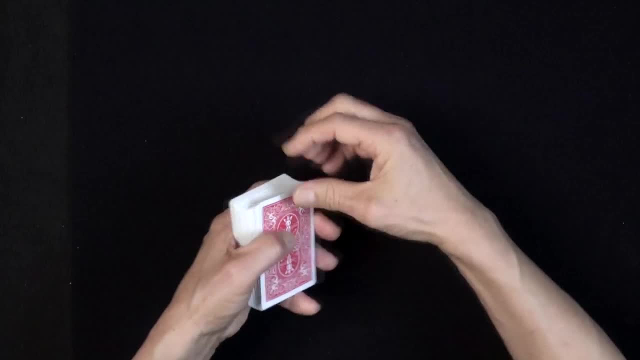 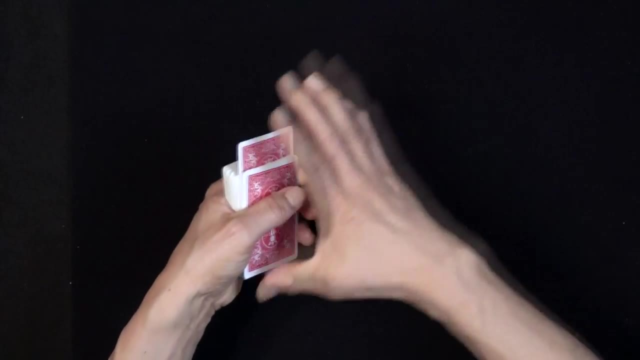 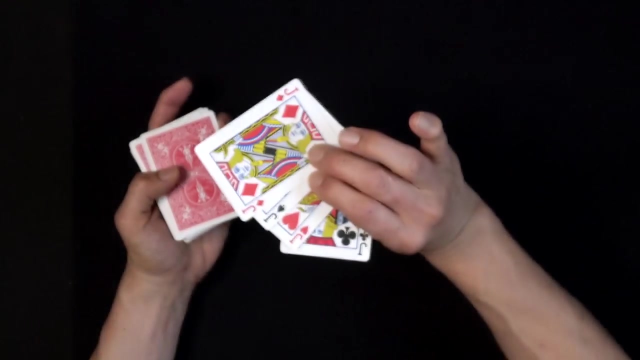 But of course that is a different card. Next one goes near the middle, But that's a different card. Finally, The last one goes in the upper third And you can show the final jack still on top, But of course the jacks are still on top of the deck. 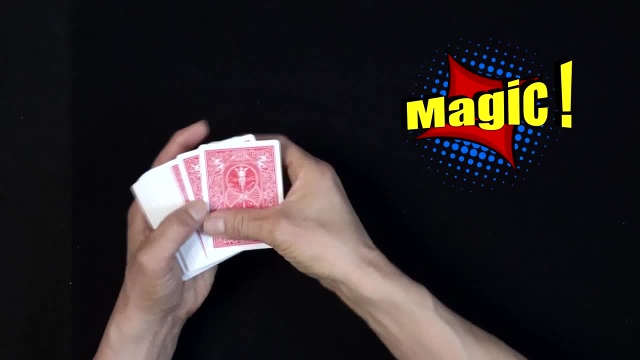 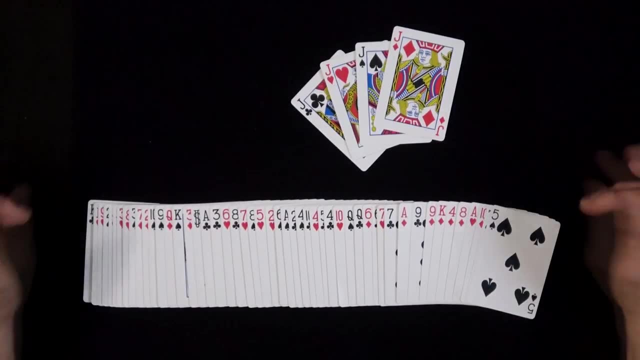 So all you do is snap your finger, do your magic wave, whatever it happens to be, And you show: the four jacks have returned. And that is a classic of magic: The four burglars, or any four of a kind that you want to work with. 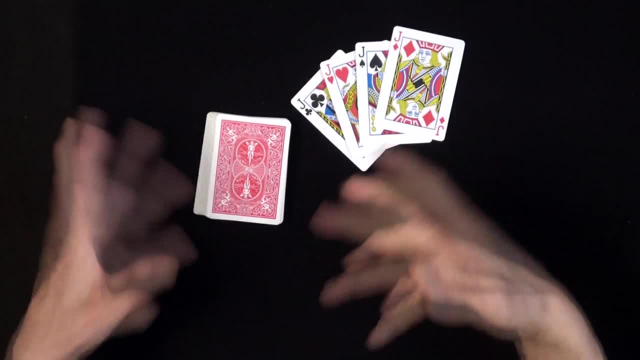 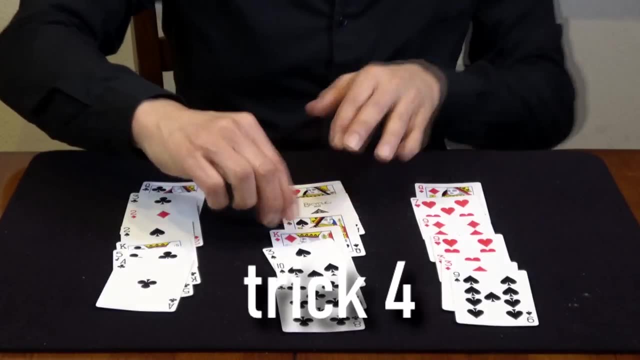 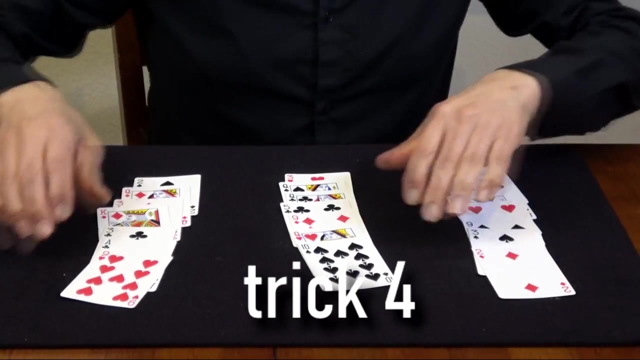 And, by the way, this is a Great trick to follow up a four ace cutting routine or production. This is a great trick for young kids And I've seen lots of kids be successful with it. You need 21 cards and it's all mathematical. 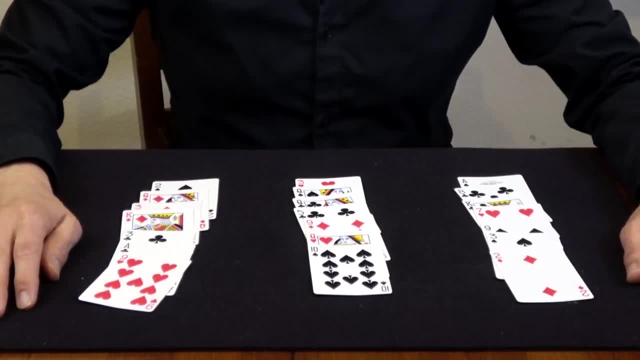 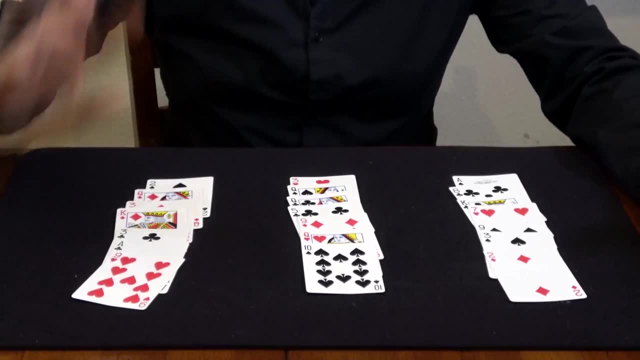 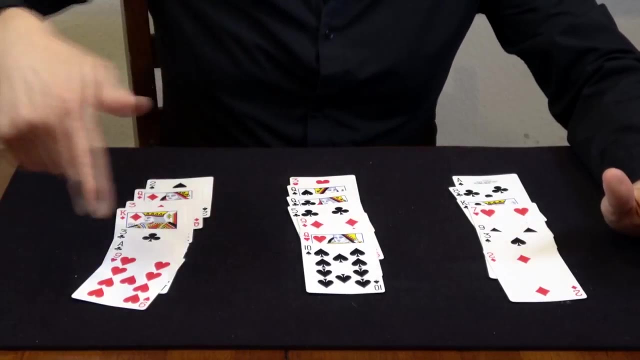 But the kids don't have to do any math, They just have to follow a certain procedure. I have 21 cards, seven in each column. So what the kid does is ask a spectator to freely select a card in their mind and then tell the kid where their card, which column their card is in. 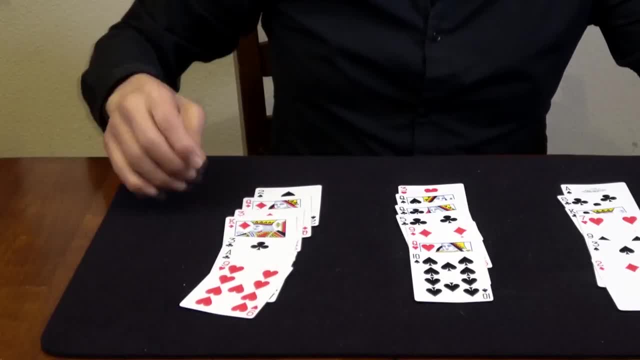 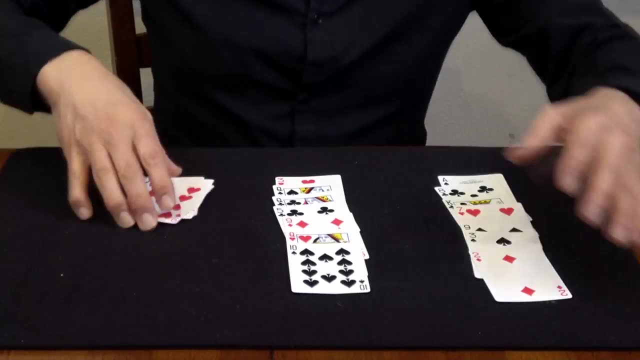 So in this case I'm going to say the spectator chose the King of Diamonds. Spectator tells the kid that their card is secretly in this column here. Now what the kid does is gather the pile, place it in the middle and place all the rest of the 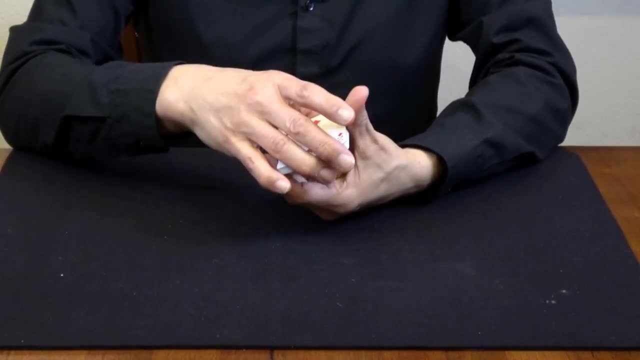 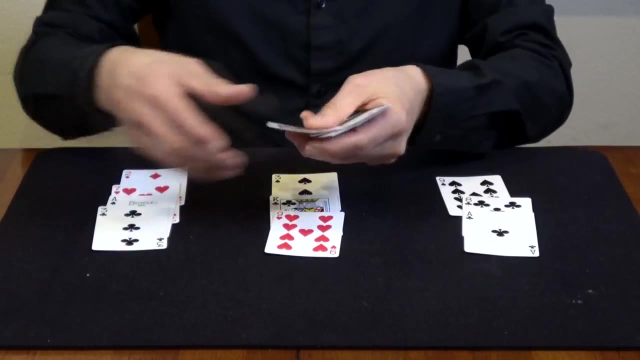 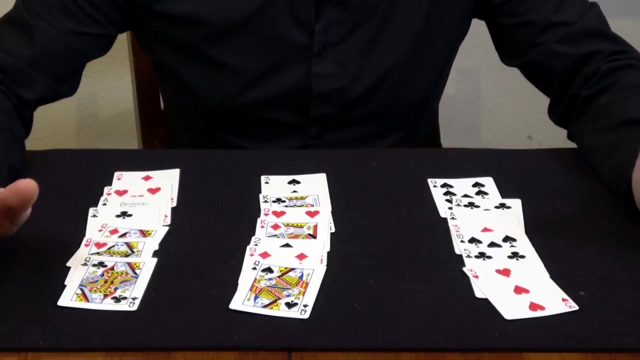 cards on top. It always goes between the other piles. Now we're going to deal the cards again. Now you have to be consistent. Notice how I'm always using the exact same pattern. Now, at this point, kid asks the spectator which column their card is in. 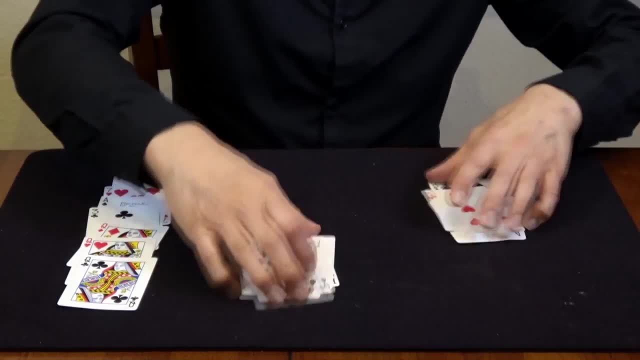 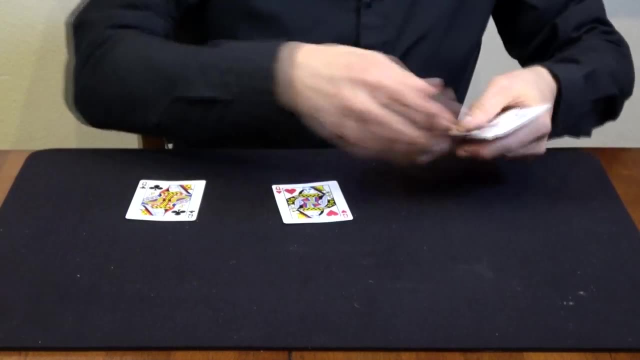 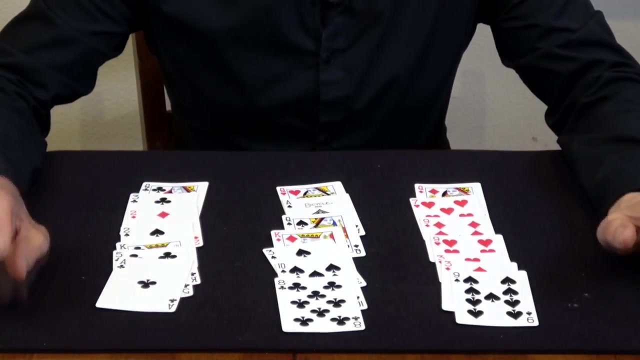 and they'll point to the middle here. There's where the King of Diamonds is, Remember. that pile goes in between the other two piles And deal once more, And at this point the kid will be able to tell the spectator what their card is. 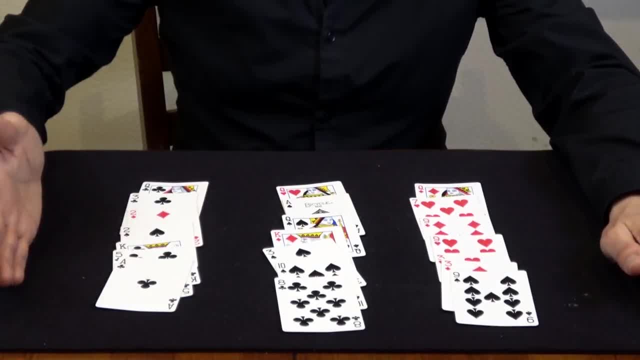 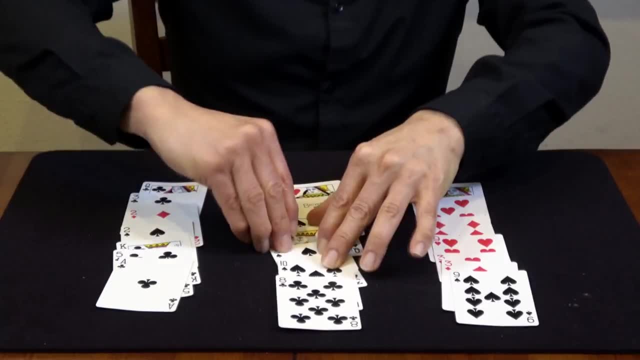 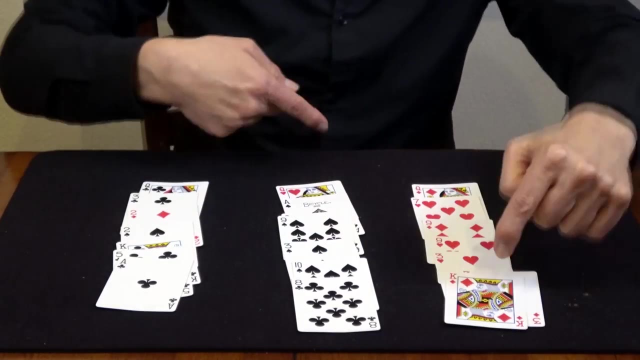 because all you have to do after the third deal onto the table is their card is in the middle column and it's always the center card, And there it is: the King of Diamonds. Now, just for fun, just for demonstration, we'll put the King of Diamonds over here. 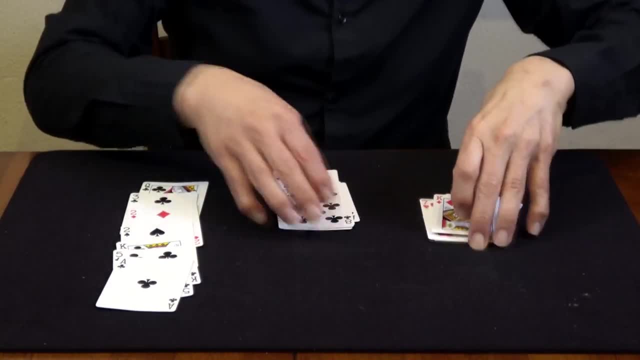 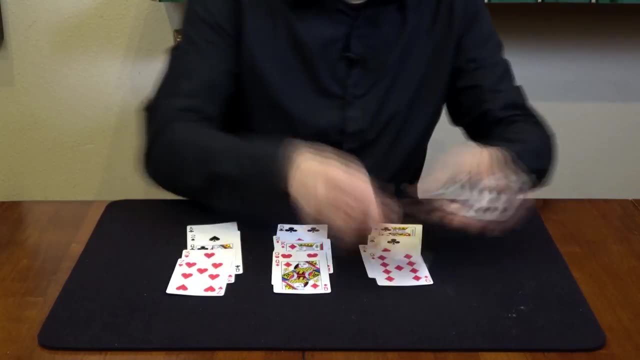 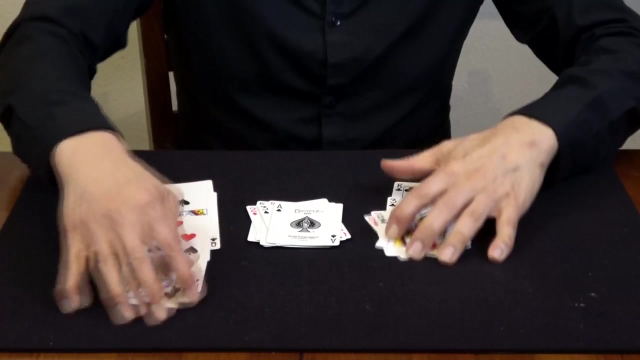 and we'll do the same process. So remember they would say their card is in this right here. Deal Spectator would point to this pile here or the column here. Remember these get gathered and that column goes in between the other two. 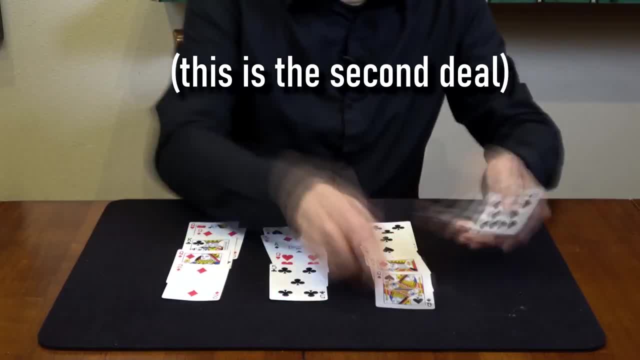 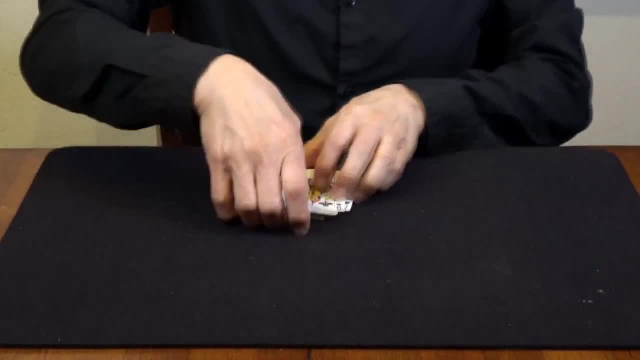 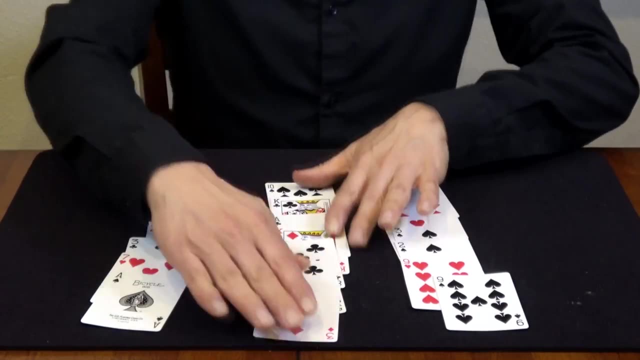 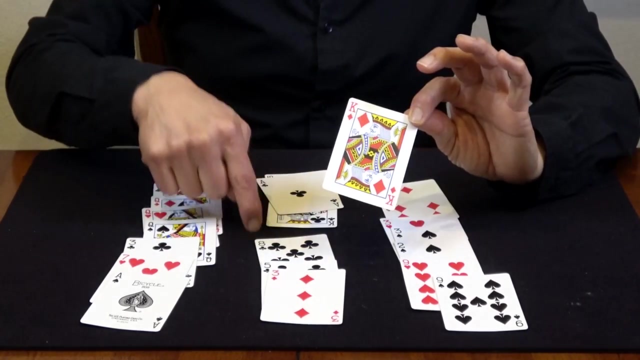 Now for the third deal. where is the card? It's right here. It goes into the middle. One more deal. I think you can see it already, Middle column after the third deal, And it's always the fourth card in the column. 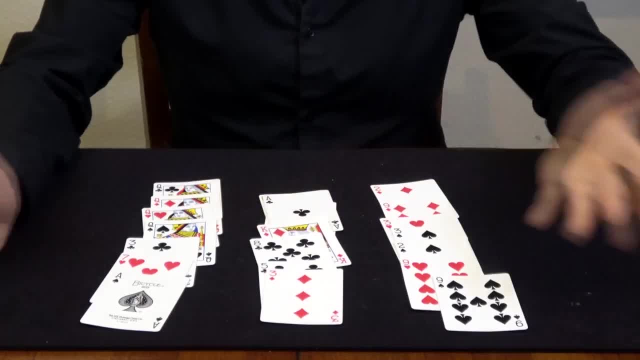 Works for any card and any starting position, So I think the kids will have fun with that one. Here's how you perform the trick. You're going to need the cards in the middle column. Here's how you perform the trick. Here's how you perform the trick. 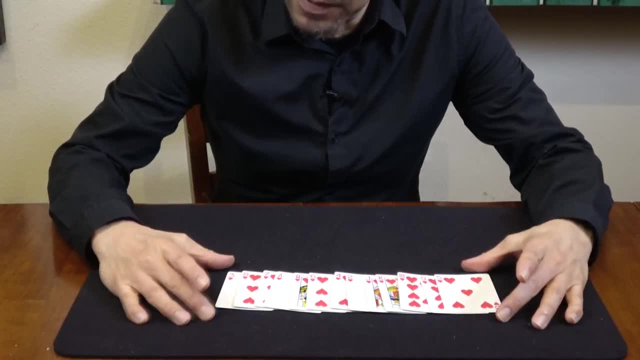 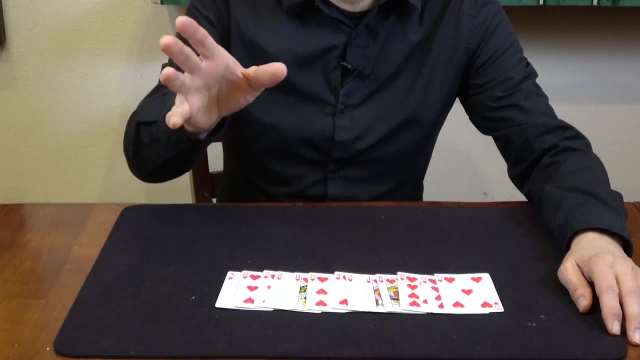 Here's how you perform the trick In a specific order, And that's the secret. And so here's the order here: Just take out the Ace through King of one suit. Line them up this way. I'll put this on the screen as well as inside the description for this video.